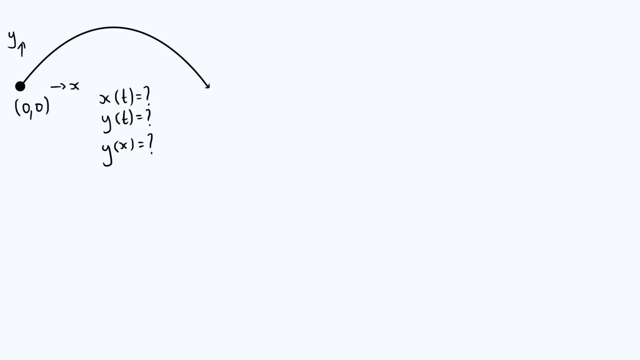 the shape of this trajectory. One is the initial speed and one is the launch angle of the projectile, Basically. so I'm going to draw on this red arrow, which is the initial velocity vector. I'm going to say length of u. in other words, the initial speed is u and this initial velocity vector is going. 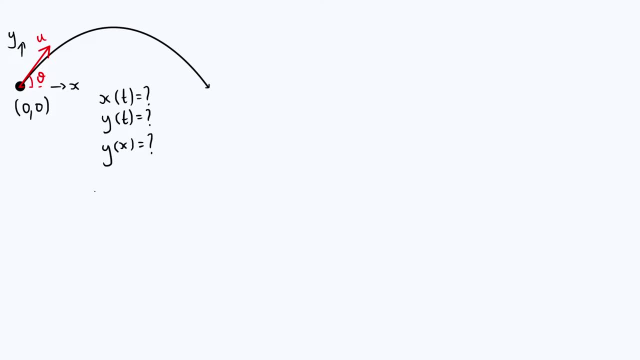 to be at an angle theta to the, the horizontal or the x direction. Okay, so let's start the analysis Now. as we often do when we're looking at two-dimensional motion, we're gonna analyze the horizontal and vertical components of that motion separately. Okay, I'm going to. 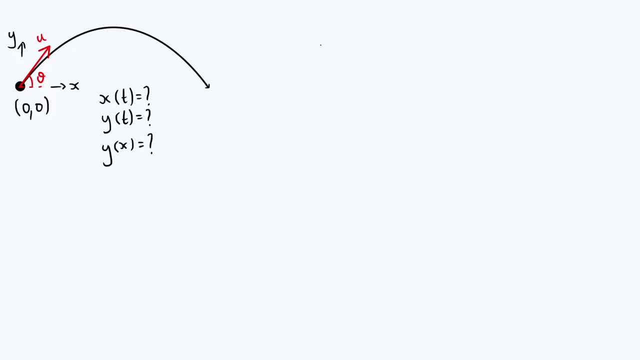 start with the horizontal component because it's a bit easier, for reasons that will become clear shortly. So, if we think about what the horizontal part of the motion is actually doing, well, there's no acceleration in the horizontal direction because there's no air resistance right. In fact, the only 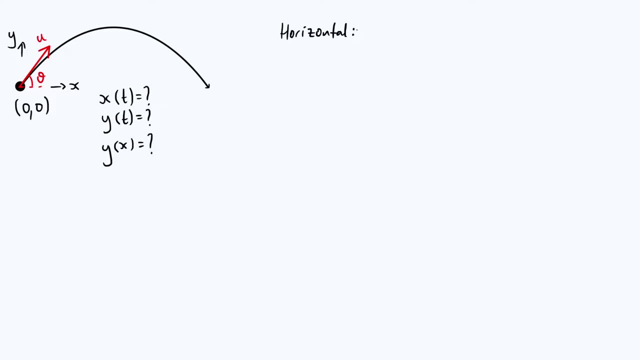 force acting on this projectile is its own weight, In other words gravity pulling it straight down and so that gravity doesn't have any horizontal component, right? So what that means is there's no acceleration, and so we can just use the simple equation: distance is equal to speed, times, time. right, because there's just no acceleration. Now, if we 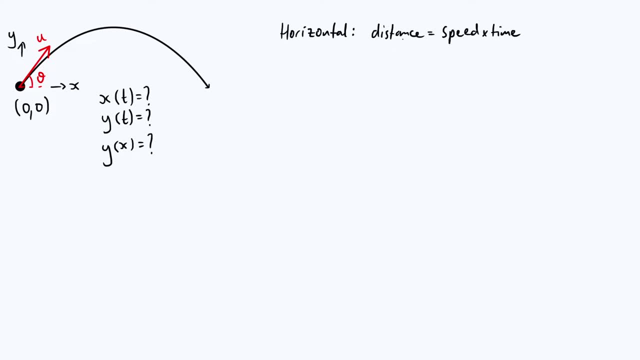 think about what these various quantities actually are. the distance in the horizontal direction, by definition, is just x, right, it's just the x coordinate. So the left hand side of this equation is going to be x. and well, what is the speed in the horizontal direction? The speed in 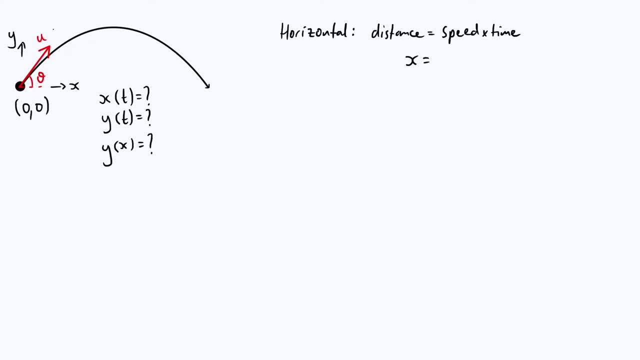 the horizontal direction is basically what you get from resolving your initial velocity vector in the x direction. right, because that component of the velocity is not going to change over time, because there's no acceleration. So I can just put here u cos theta, because that's the horizontal. 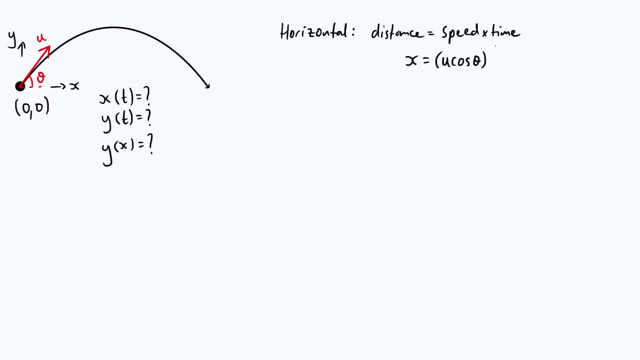 part of that initial velocity vector, all right. and the time? well, that's just what I've called t, right. So there you go this thing here. x equals u cos theta times. t is just an equation of motion that describes how the x coordinate changes with time. it just increases linearly. So I'm going to 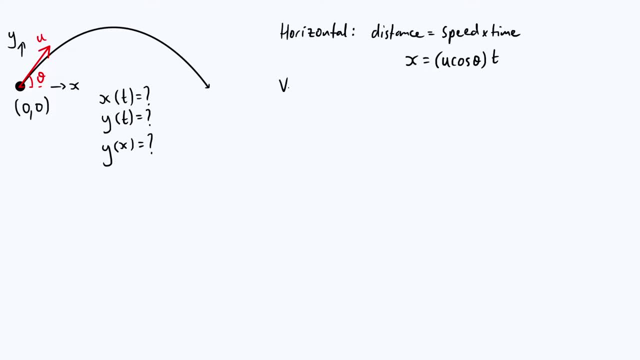 just put here u cos theta times t is just an equation of motion that describes how the x coordinate changes with time. it just increases linearly, Okay. so what about the vertical direction? It's going to be slightly more complicated because of the force of gravity, which is acting in the 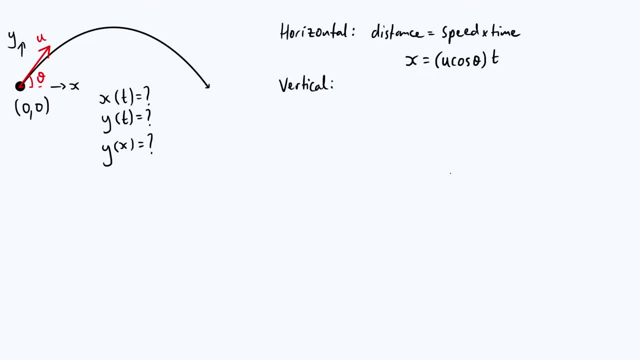 vertical direction. Now the good news is that it's if we assume, if we neglect the variation of the gravitational field strength with height above the surface of the earth or whatever planet we're on which we usually can on reasonable scales, then the acceleration is going to be constant. 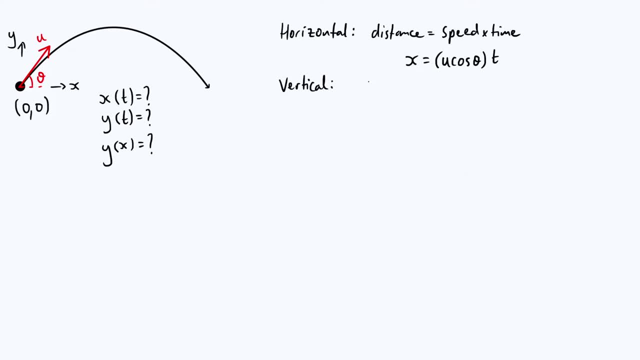 Right, and that means we can use the constant acceleration equations or the suvat equations. and when I'm doing that, I usually start by just writing out all these letters- s, u, v, a and t- and think about which ones we actually know. And so s is the displacement, u is the initial. 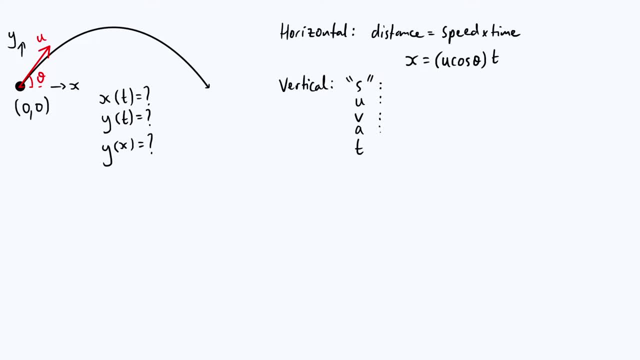 velocity v is the final velocity, a is the acceleration and t is of course still the time. Now, by definition of the y coordinate, the displacement in the vertical direction is just the acceleration of the velocity. So if I take the y coordinate and I take the velocity of the, 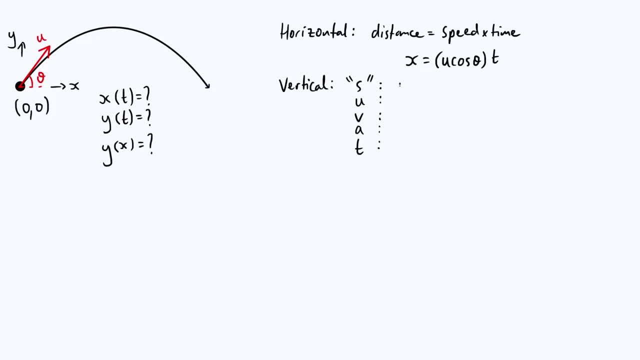 y coordinate and I take the velocity of the velocity. So if I take the velocity of the velocity right, so this s in suvat is now really just just y. Okay, what's u? well, u is really the vertical component of the initial velocity. We already found the horizontal component earlier on that. 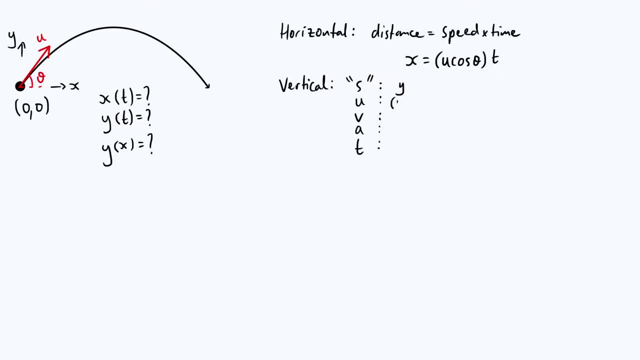 was u cos theta. so the vertical component is just going to be: well, we need a sine instead of a cos, so that's going to be u sine theta. In fact, I don't even need the brackets there, so I'll just put that as u sine theta, Okay. 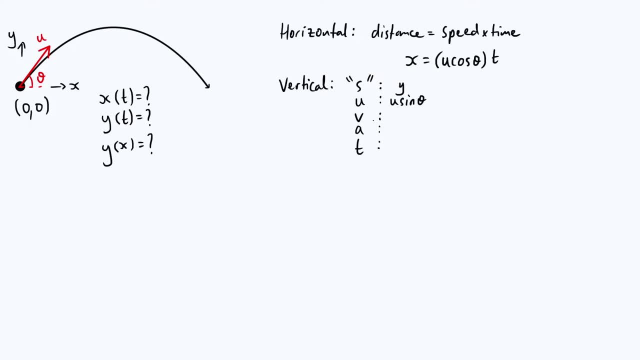 The final velocity v. well, without doing more calculations, we don't really have a way of directly saying what that final velocity is, and so I'm just going to leave that blank. The acceleration, that's just the acceleration due to gravity, and so it's going to be usually. 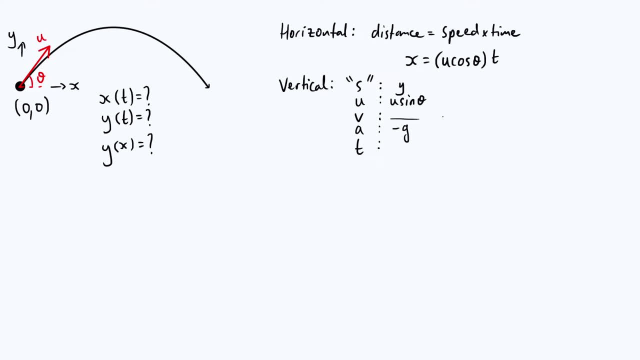 written as g, but it's really minus g because I've defined y to be increasing in the upwards direction and gravity is of course pointing downwards and t is still just the time, so I'm just going to put a t there, Right, and so we know s? u, a and t and the suvat equation that links all of those quantities. 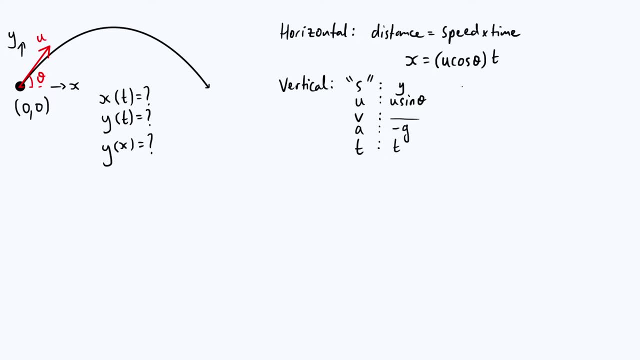 together, without saying anything about v, is this one s equals u t plus a half a t squared. Okay. so let's see what happens if we kind of put all of these values into that suvat equation. Well, s was y, so we get y equals the. u is really um. u sine theta uh, so we get u sine theta t. 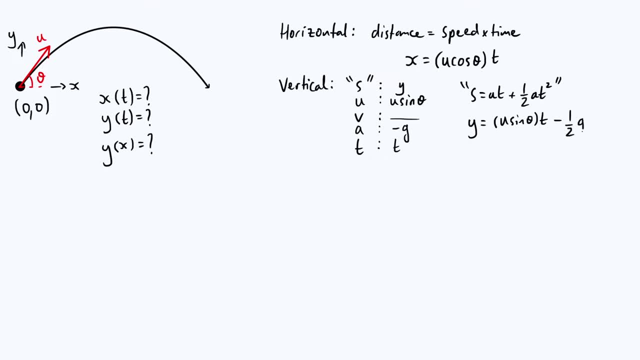 and then we're going to put a t there, So we're going to get minus a half g t. squared, minus is just because, well, the acceleration itself was negative. so there you go. there is a parametric equation for the y coordinate as a function of time, right? so I'm just going to label these two parametric equations. one: 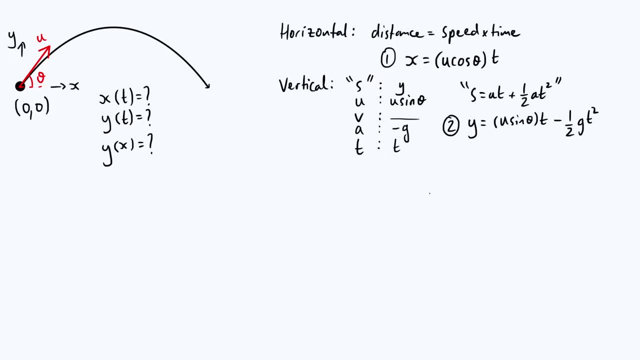 and two. Okay, so we've achieved our first goal, which was to find those parametric equations. now let's see if we can combine them together to eliminate time and just get the cartesian equation of that trajectory. So fortunately, we've got a parametric equation, and we've got a parametric equation and we've 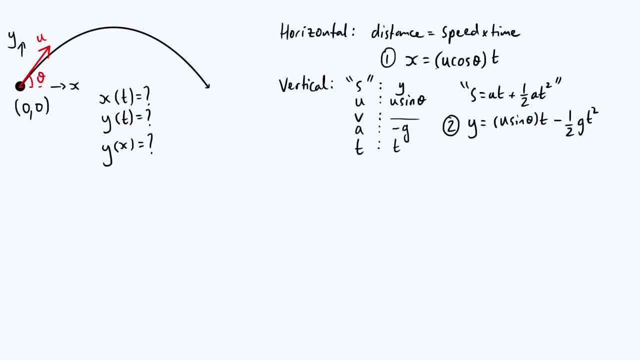 got a t squared equation. So basically we can rearrange equation one fairly easily to get t as the subject um, and then just substitute that into equation two. So I'm going to say basically we just want to substitute the equation uh one into equation two. 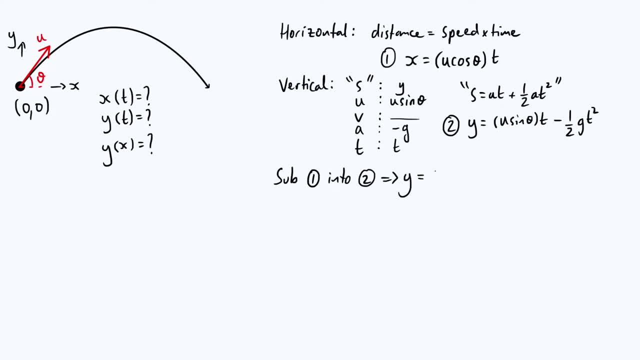 uh, what's going to happen if we do that? well, we still have y equals on the left hand side. um, we're going to get u sine theta. but if we rearrange equation one, we're dividing by u cos theta, and so this t is really x over u cos theta, right? So here I can just put x over u cos theta. Now I've still 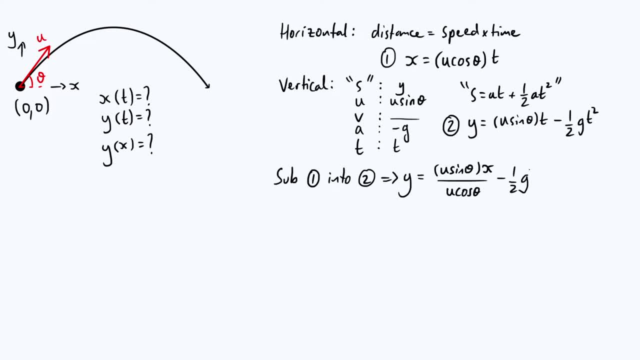 got this half g, but then I'm just squaring that entire expression for t, which was x over u cos theta, So I can just put x over u cos theta here and square that right Now. what we've got to do is simplify that as much as possible. We can use a trig identity that sine theta over cos theta is. 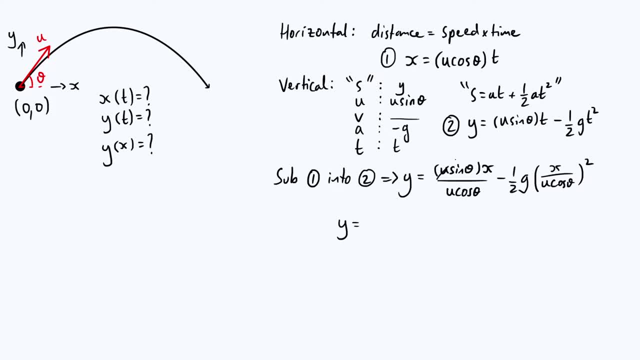 tan theta. And also in this first fraction the u's on the top and the bottom cancel out right, So that first term just becomes tan theta. So we get y equals tan theta x, And then I'm just going to well, expand out the brackets and write that as just one fraction. Second term is going to be: 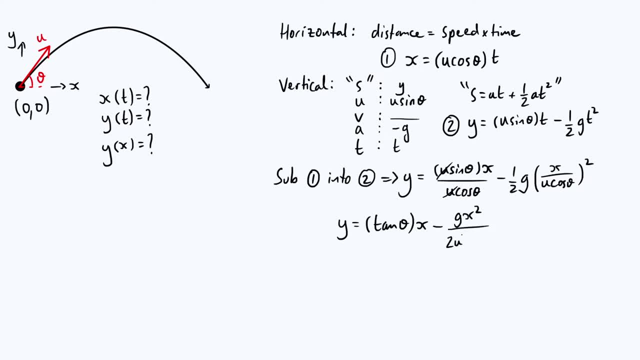 minus gx squared over Two, u squared cos squared theta, And there we go. There is our Cartesian equation of that trajectory. So it's just a. it's an upside down quadratic. Basically it's we would call it a parabola, right? So it's got this nice symmetrical shape, which is because, again, we've got no air. 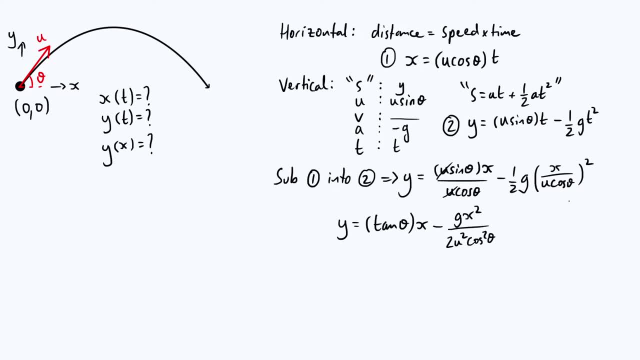 resistance. Now we can use that Cartesian equation to get an expression for the range of the projectile, because the range is defined as the maximum horizontal distance that the projectile is at, And so we can use that to get an expression for the range of the projectile. 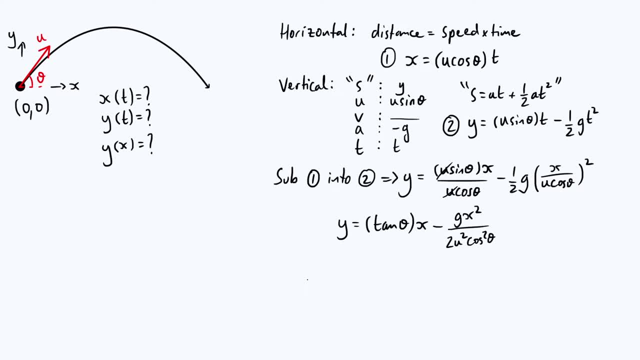 And so, assuming that the ground is perfectly flat, that means we're looking for the x-coordinate at the point where the y-coordinate is zero. right, Because when it hits the ground it doesn't. its height has just reduced back to zero. So what we're essentially doing is setting 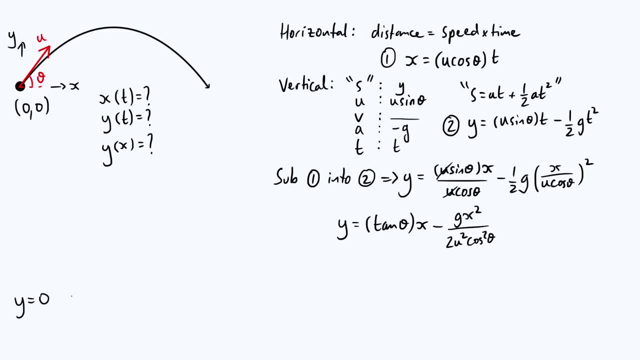 y to be zero. So I'm going to say y equals zero, and let's substitute that into our Cartesian equation and see what happens. So first thing I'm going to say is: well, it's a quadratic, The expression for y is a quadratic right, And so we want to factorize it, if we can. Fortunately, 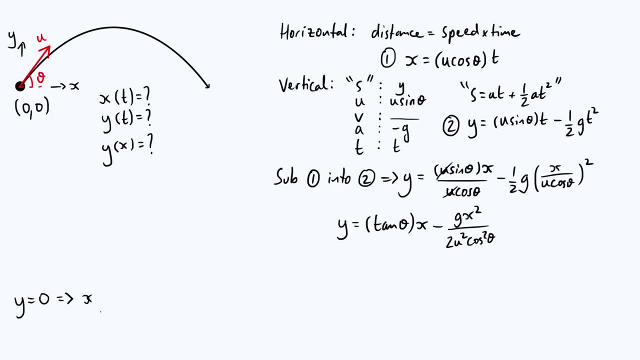 we can, because we can just take out an x. So I'm going to say x and then brackets, tan theta, and then we're going to get gx over 2u squared cos squared theta. That whole thing is supposed to be zero if y is zero. And there's two solutions to this right. One of them is just: x equals zero. 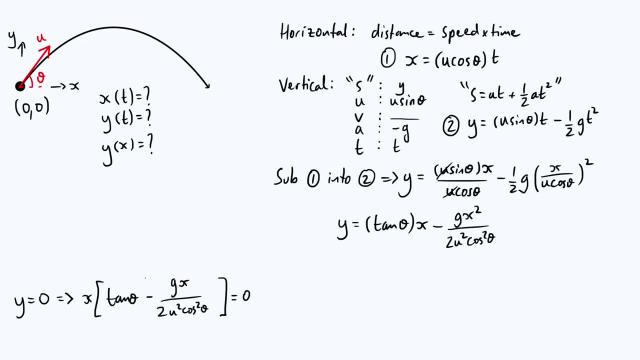 which makes sense because that corresponds to the starting point of the projectile right, Because it starts at coordinates x equals zero and y equals zero. So that's the solution that comes from this x in front of the brackets. The more interesting one is a solution we get by setting. 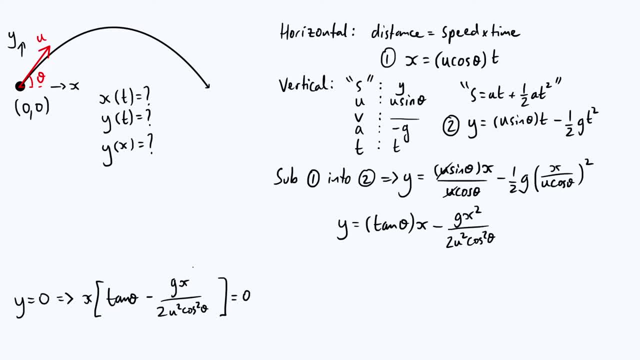 the entire bracketed term to zero And that is going to be the range right, Because that's the other point on the trajectory at which the height reduces to zero. So this x here we could call that capital R for for range. and so if we just require the entire bracketed term to be zero and we rearrange that,